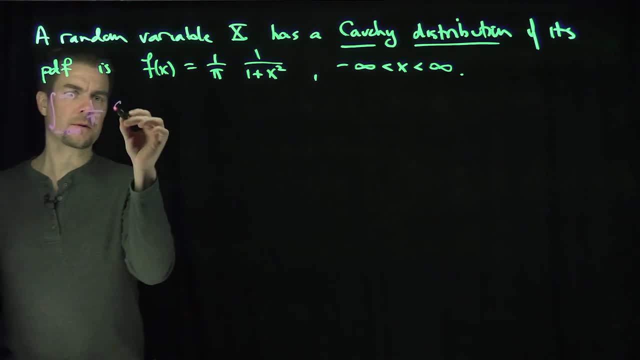 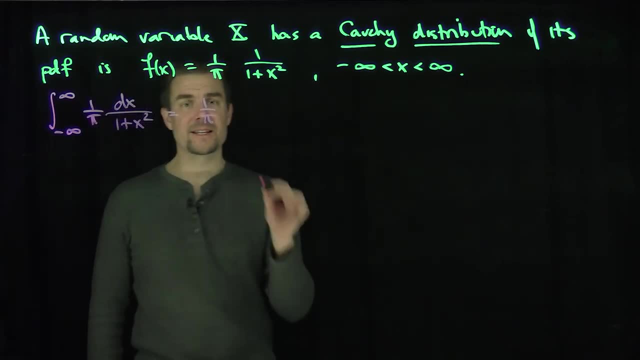 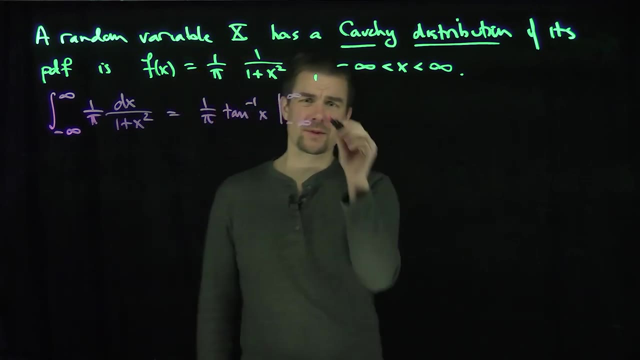 infinity to infinity, of one over Pi, dx over one plus X squared, I get a one over Pi and an antiderivative of one over one plus X squared is tangent inverse. Tangent inverse of X evaluated from negative infinity to infinity, and taking limits here when I'm doing this, but sort. 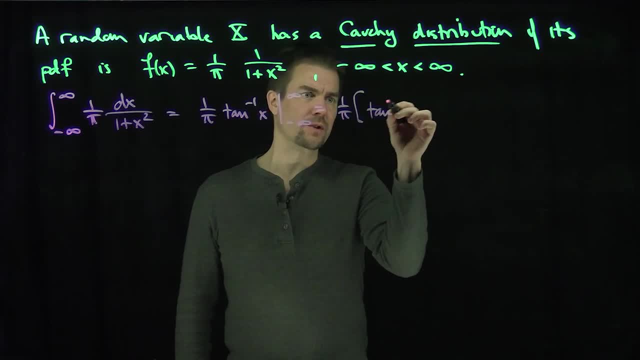 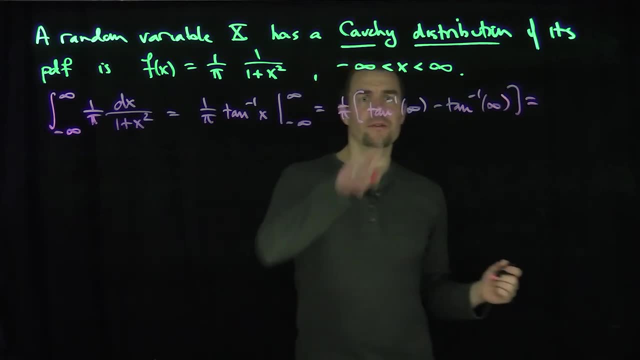 of. we can note that I'm going to have a tangent inverse of what? A tangent inverse of positive infinity minus tangent inverse of negative infinity. And the tangent inverse of positive infinity is Pi over two, and this is negative Pi over two, so I get a total factor of one. 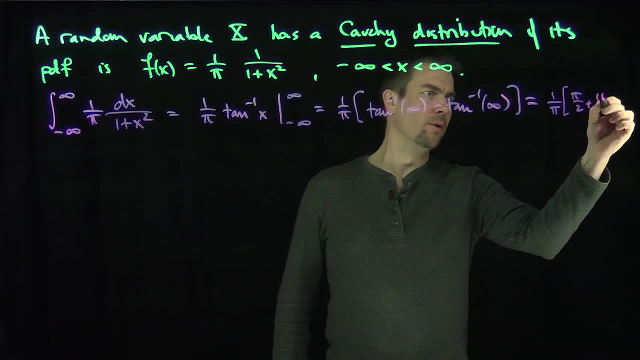 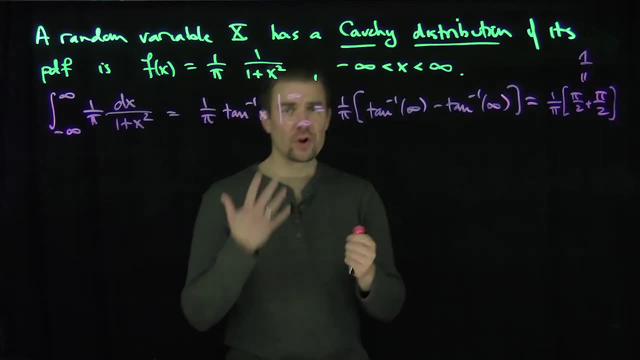 over Pi, and then Pi over two plus Pi over two. So we do indeed see that this is equal to one and we do have a valid pdf. now we can use this same formula to find the cumulative distribution function of a cauchy distribution. so let's do so. so the cdf. 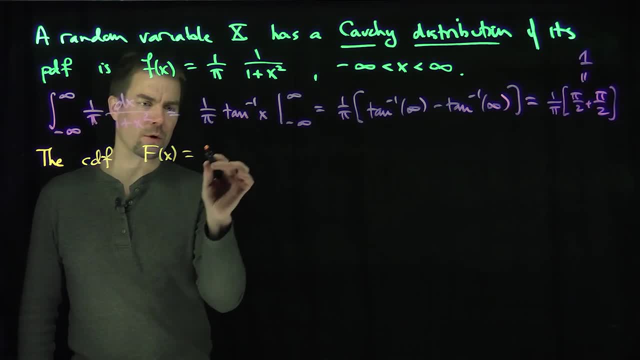 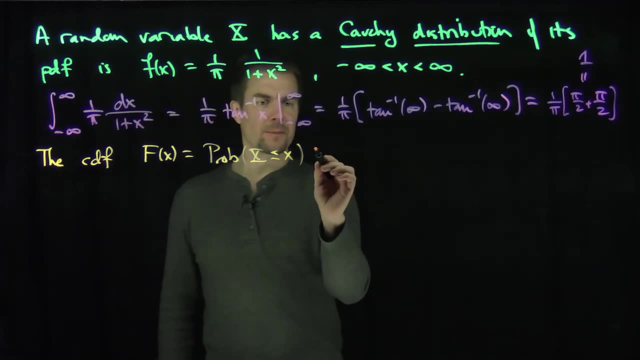 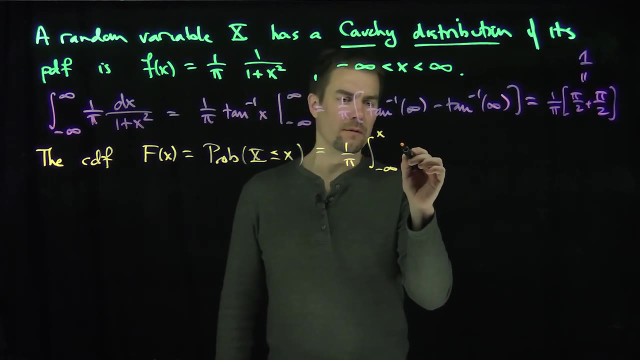 is found by the following ways: f, capital of x, and that's of course just the probability that x is less than or equal to little x. okay, and so this is going to be 1 over pi, 1 over pi, and then the integral from negative infinity up to x, of what of dt over 1 plus t squared. i have to. 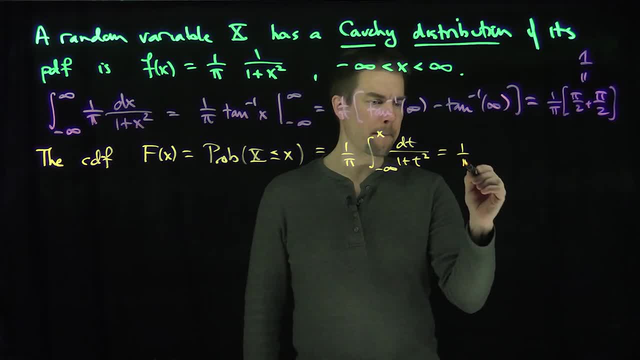 introduce a dummy variable now, and so this is what this is: 1 over pi, 1 over pi, and then tangent inverse of x, tangent inverse of x minus, tangent inverse of negative infinity, which is negative, negative. pi over 2. so plus a pi over 2, right? so we have over here for. 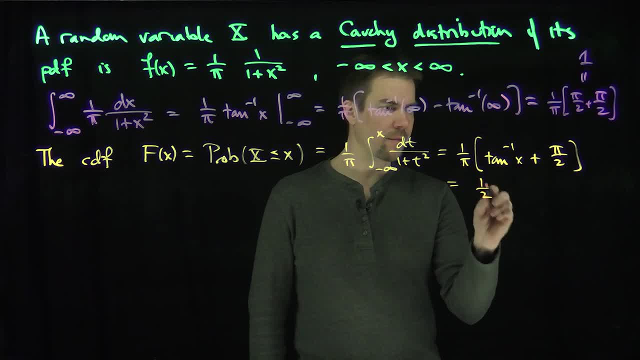 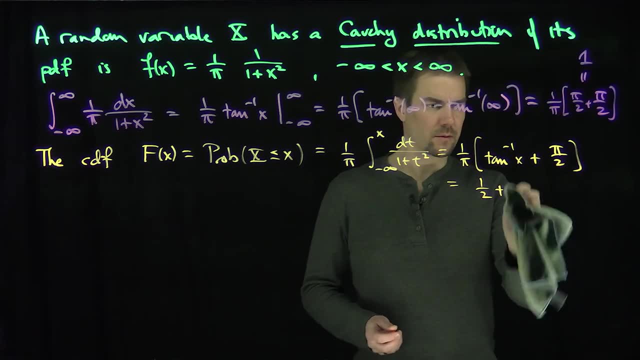 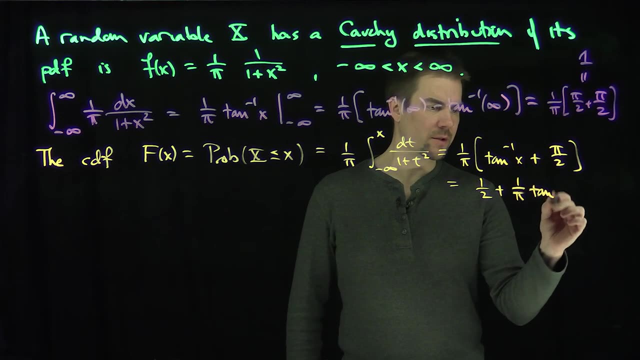 the cdf is what the cdf is going to be, what the one? this is going to be a one half, and then plus tangent inverse, plus 1 over pi, tangent inverse of x. okay, okay, so plus 1 over pi, tangent inverse of x. okay, now, clearly, as x goes to negative infinity, what's? 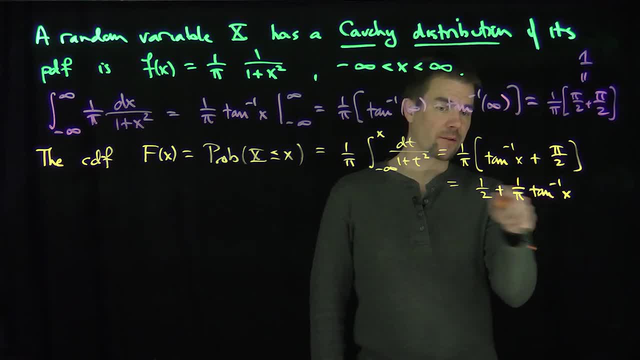 happening is going to negative pi over 2, so that's going to go to 0. when x goes to infinity, it's going to pi over 2, so i get to 1. so this isn't indeed a valid cdf. so that's what the cdf is. 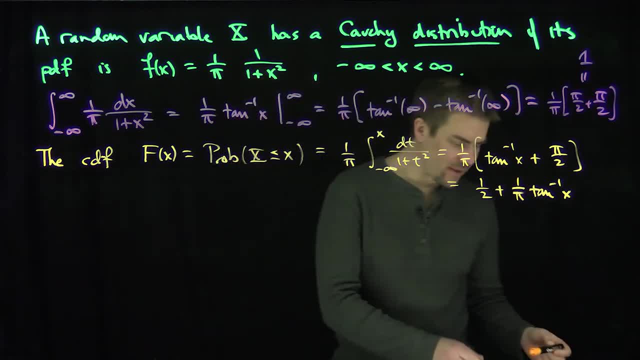 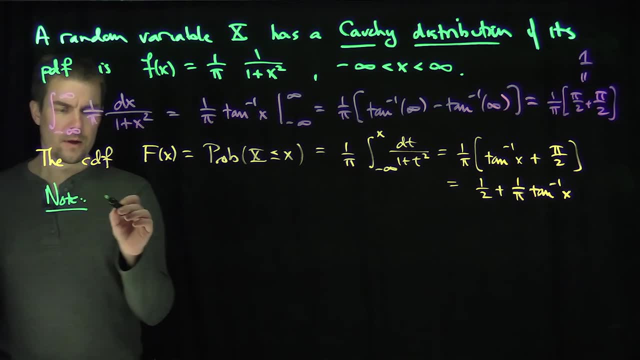 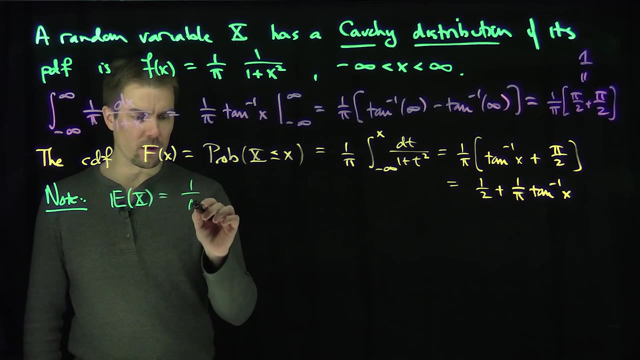 right, and so now let's make a note about this. one note that happens is that the moments of these random variables do not exist, right, so the moments? just as a note, the expected value, for example, of x would be what would be this integral over here, 1 over pi, the integral from negative infinity to infinity of what, of x over 1 plus x. 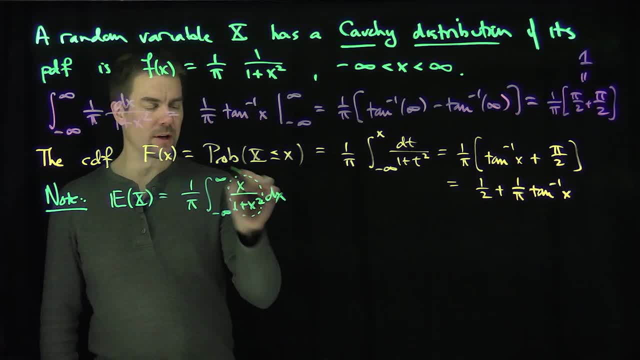 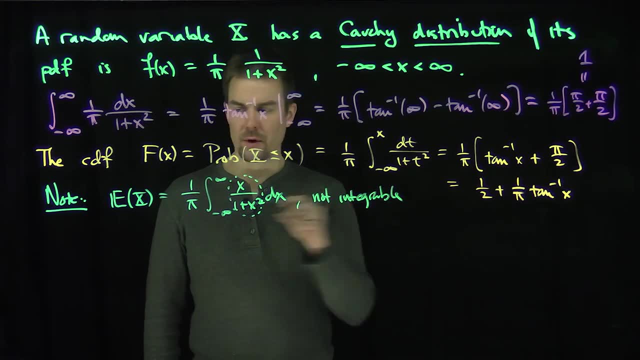 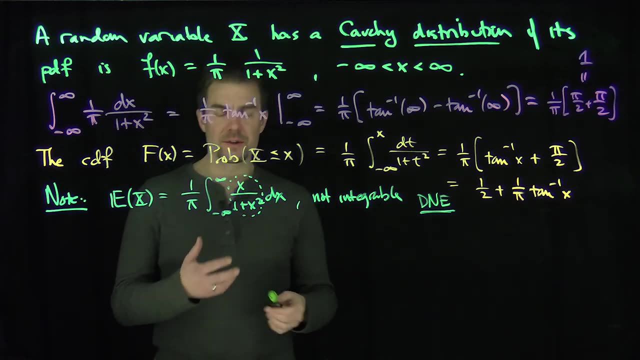 squared dx and this function over here is not absolutely integrable, right? so this is not integrable function. this is not integrable and so this expected value does not exist. the same is true for any higher moments. so the expected values does not exist for this cauchy distribution. and of course, we can see this because, as i take, 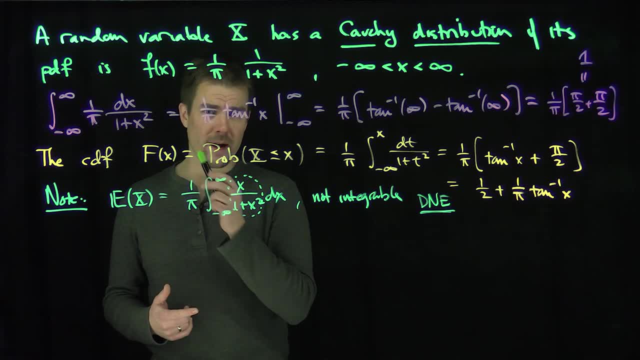 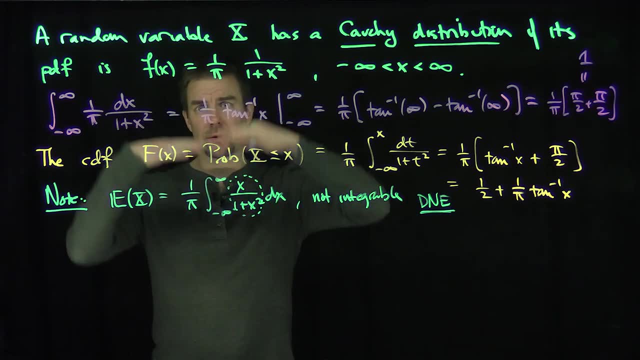 different limits, as i let one variable go to negative infinity and the other variable go to positive infinity. this term over here looks like a logarithm and the logarithm does not converge. as we go to infinity we're going to have a we're at different scales this thing can give. 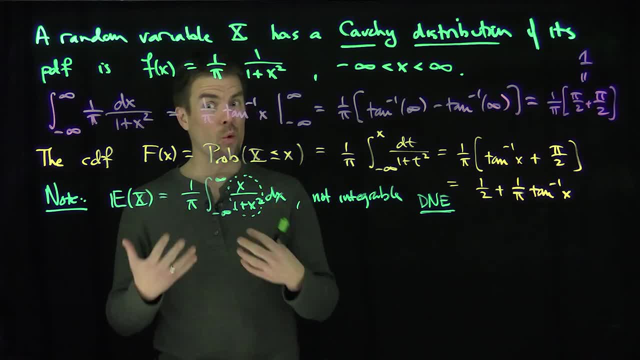 me different limits. so this limit does not exist because this function over here is not an l1 function, absolutely integral function. so the moments of cauchy- random variables do not integrate- exist. so the first moment doesn't exist, the second one doesn't exist for the same reason. 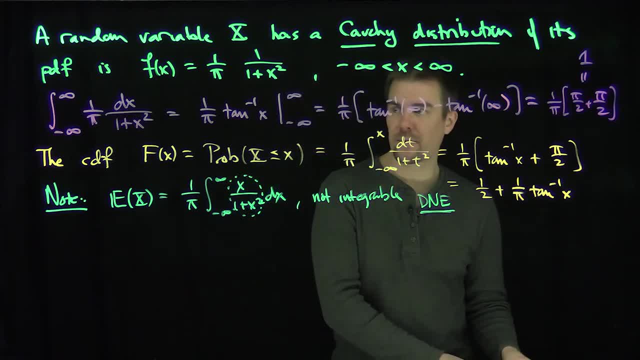 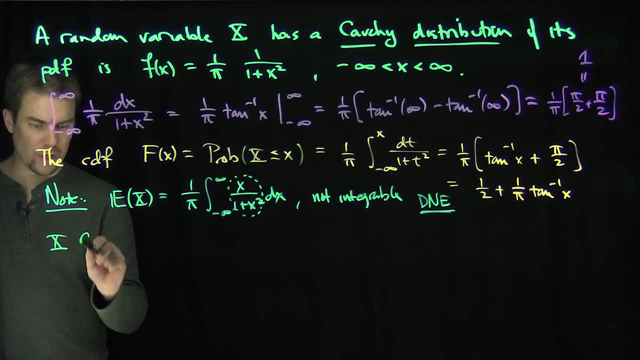 all the higher moments don't exist for quotient random variables, but they do satisfy a beautiful property. and there's one beautiful property of these things, and that what i'd like to do is i'd like to consider if x is cauchy, so i'll say x is cauchy, and if i look at a random variable, if i 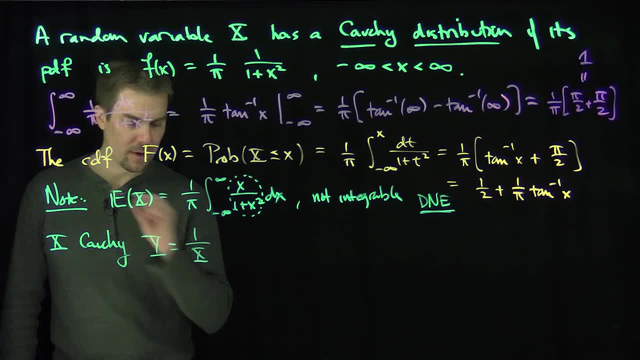 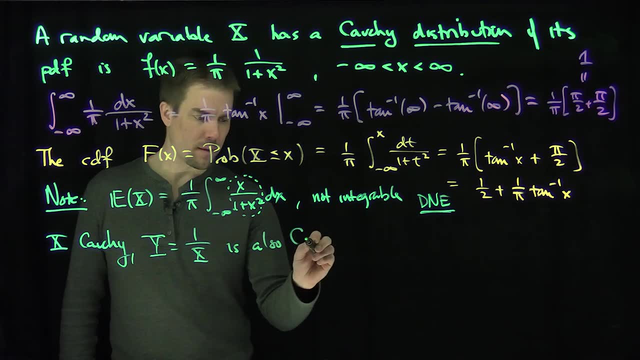 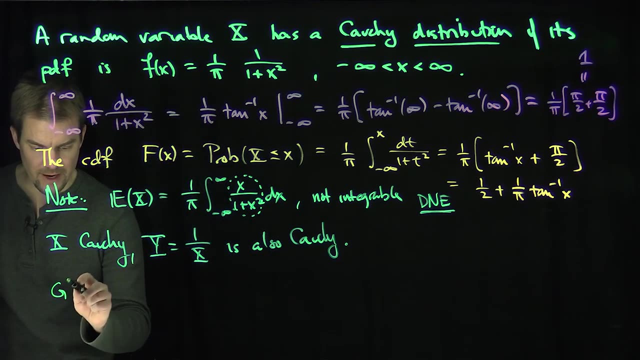 look at y, which is 1 over x, then i want to find the distribution of y is also cauchy. okay, let's prove that. so how do i prove that? well, i'm going to consider the cdf for y. so let's let g of x. 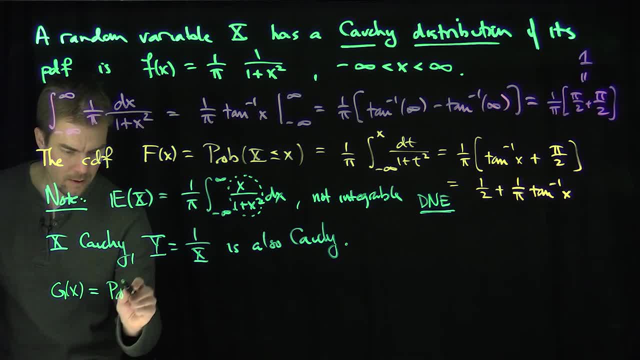 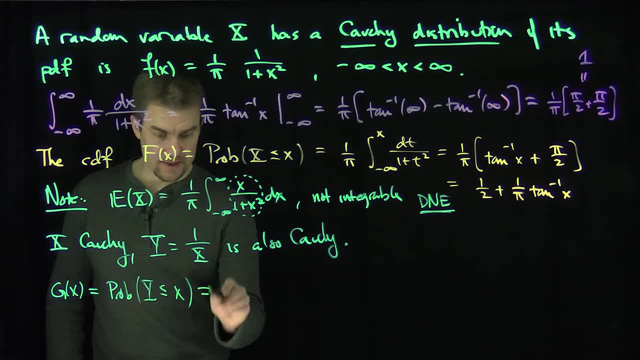 be the cdf for y. so that's the probability that y is less than or equal to x. well, if y is less than or equal to x, that says that's the exact same thing as saying that that's the exact same as the probability that one that x itself is bigger than or equal to one over x, by taking the.